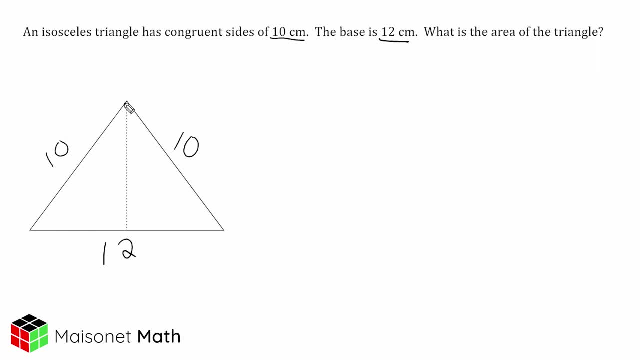 base length right here, slightly longer than each of these two congruent sides right here, And we have to use this information to figure out the area of the triangle. Now remember: to find the area of any triangle, we simply take the base of the triangle, multiply by its height. 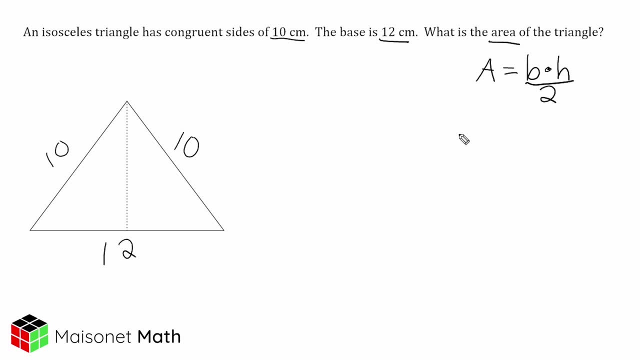 and then divide that product by two. Now the base of the triangle is given- it is 12, but the height of this triangle is not given. We have to use this information to figure out what this height is. So what we're going to do is we're going to see that this height right here. 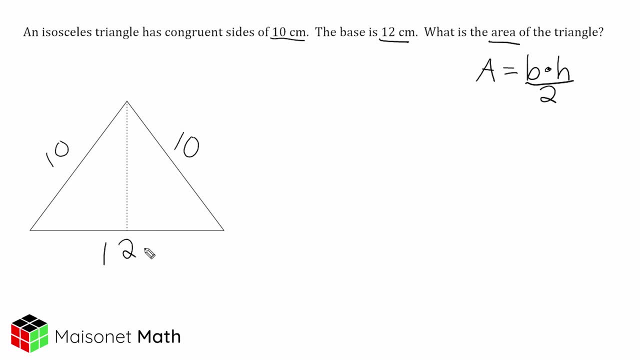 divides this isosceles triangle in half, We have two congruent right triangles. So if we just take a look at this triangle right here, we can see that the height of this triangle and half of this base form the two legs of our right triangle. So what we need to do is figure out what is the 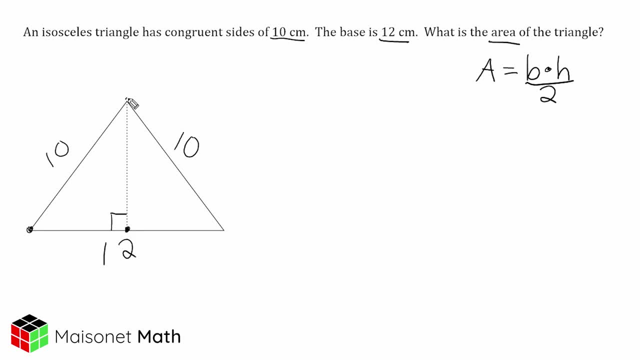 distance from here to here, And then we can see that the height of this triangle is divided by two. We can use the Pythagorean theorem to figure out what this unknown height is. Now, because this triangle is divided perfectly into two equal parts, we know that we can take 12 and divide 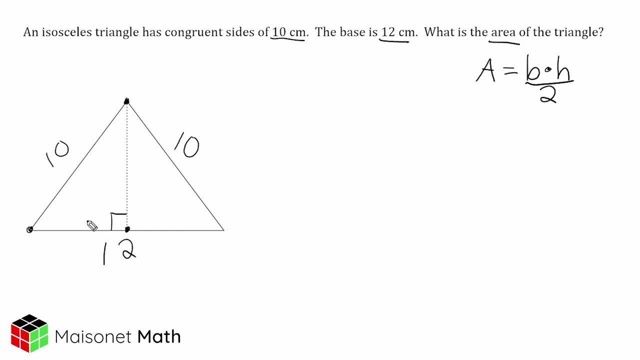 that by two, which is six. So the distance from this point to this point is six centimeters, as is the distance from this point to this point. But all we really have to do is take a look at one of these two triangles. So what we're going to do is take advantage of the Pythagorean theorem. 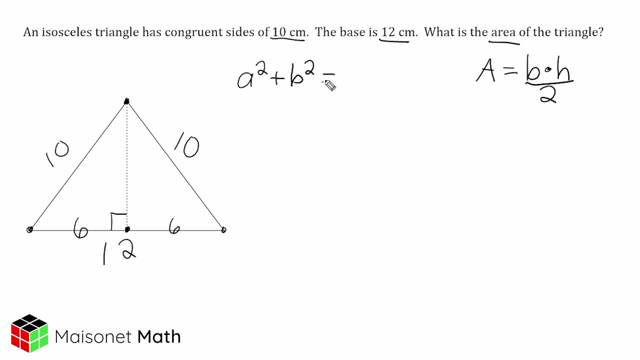 consider that one over the square, extract that one over here, subtract the total line and write that one over there, And the posted by the Pythagorean theorem is approximately six centimeters, plus that one over here, minus volume here, And that divided by two equals four centimeters. 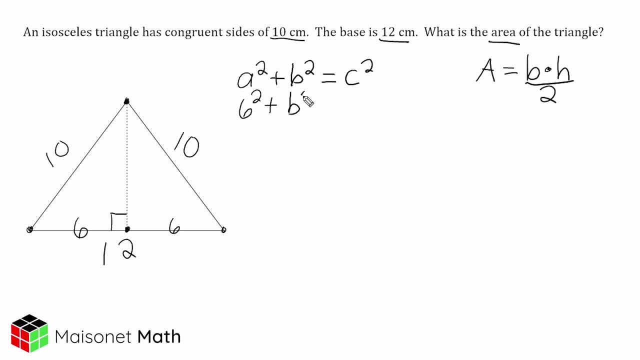 So that one over here and subtract all that minusほど equals combinily Hindi Extruded. there's a whole bunch of numbers derived out of number threeраф mk. If you left off with two, youית put them back together two times threeanimals. Now, if you just exclude those in this, 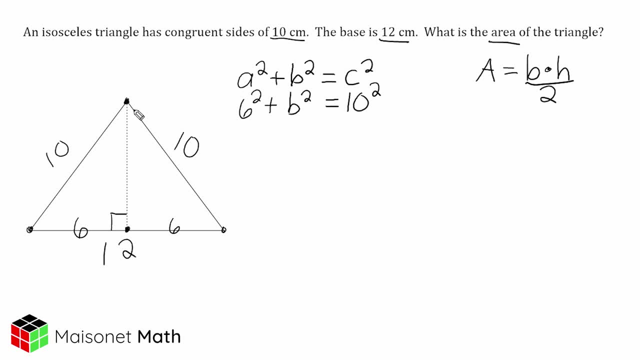 solve for the length of B And that will tell us what the height is. And once we have the height we can plug it into our formula right here to figure out the area of our triangle. So let's take 6 and square that, That's going to be 36 plus B squared equals 10 squared, which is: 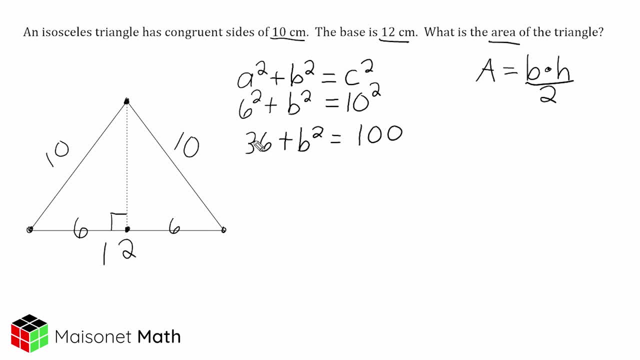 100. Then we're going to take this positive 36 and move it to the other side of our equation, So we're going to subtract 36 from 100. And that ends up giving us 64. And now we have just B squared remaining. Now B is not by itself, yet We have to remove the. 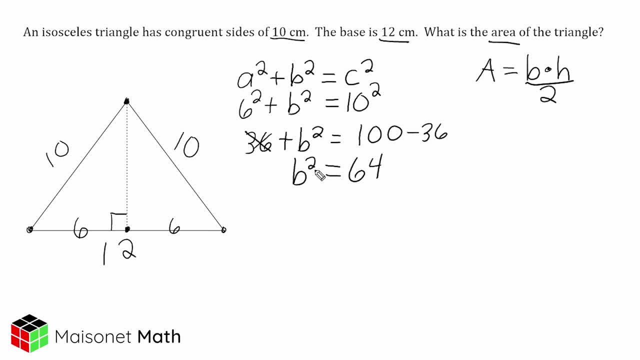 exponent of 2.. And the opposite of squaring something is to square root something. So if we put a square root symbol over this, the exponent of 2 and the radical symbol will cancel each other out, leaving us with B. And to balance our equation, we take the square root of 64,. 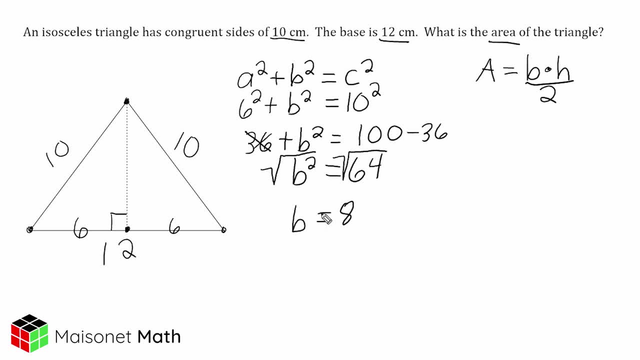 which is equal to 8.. So now we know that the length of this height is 8 centimeters. So now what we can do is go over here to our area formula And we can plug in the length of the original base of the entire triangle. 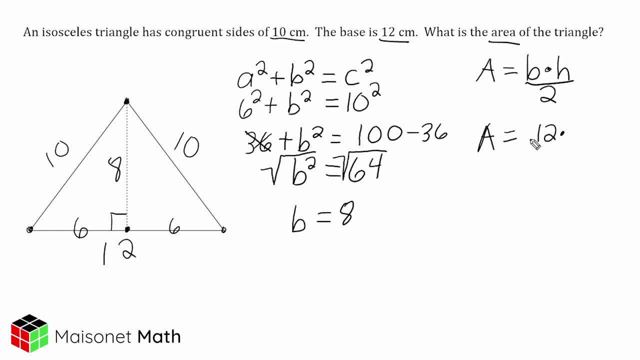 which is 12.. Multiply that by our height, which we just determined is 8., And then divide that by 2.. So what we can do now is we can take 12. times 8,, which is 96.. And divide that into two parts, And that would give us 48 square centimeters. 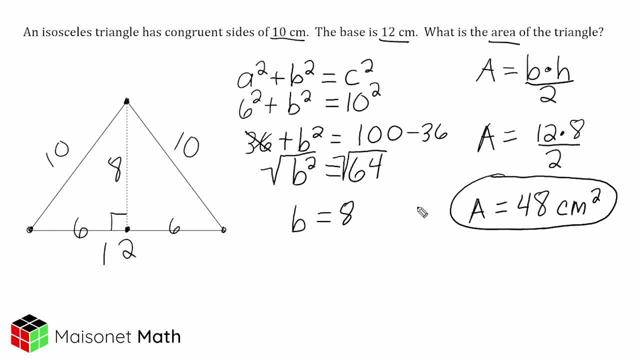 So what we had to do to find the area of this triangle is we had to take advantage of the Pythagorean theorem to figure out the unknown height of this triangle. And once we determined what that height is, we plugged it into our area formula and solved. 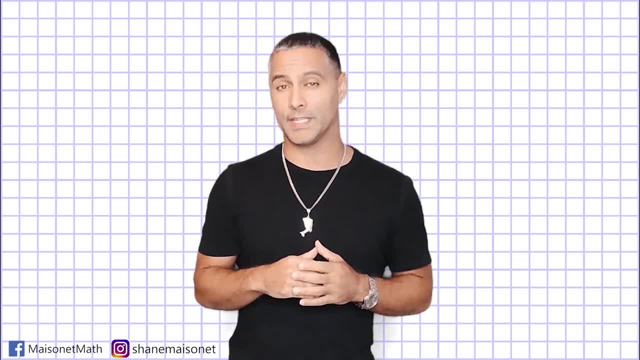 Hey, I just want to say thanks for checking out this math tutorial. Please don't forget to hit that subscription button and enable notifications so you can be informed as I upload new math tutorials to my math channel. Until next time, this is Shane Masonet with Masonet Math. Thanks for watching.